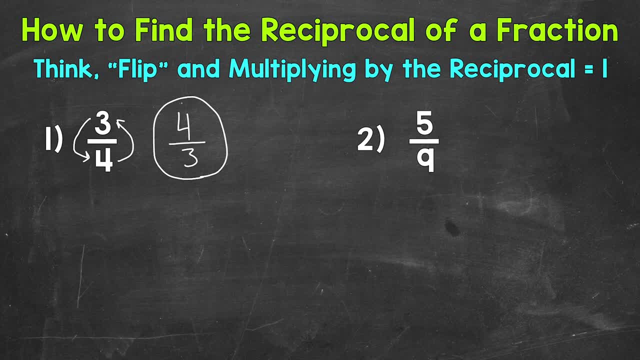 Now let's multiply our fraction by that reciprocal to show that we get 1 when multiplying by a reciprocal, So 3, fourths our fraction, multiplied by the reciprocal of 4 thirds. So multiply straight across Numerators: 3 times 4 is 12.. Denominators: 4 times 3 is 12.. So same numerator, same denominator. 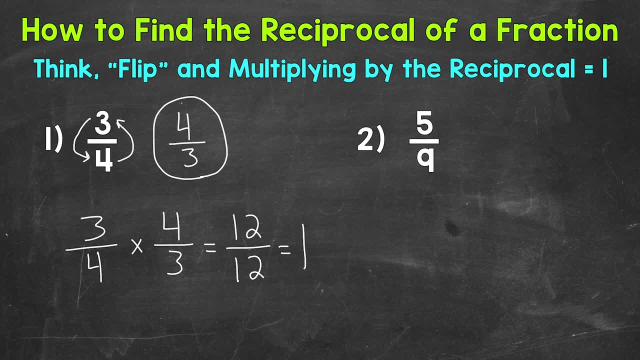 that equals 4.. 1. So again, the reciprocal of 3 fourths is 4 thirds. Let's move on to number 2, where we have 5 ninths. So again, let's flip the fraction to get the reciprocal. 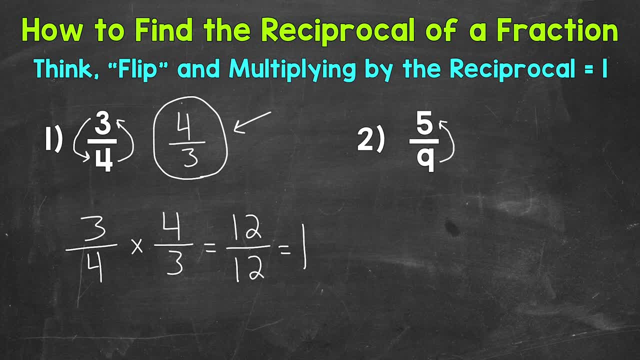 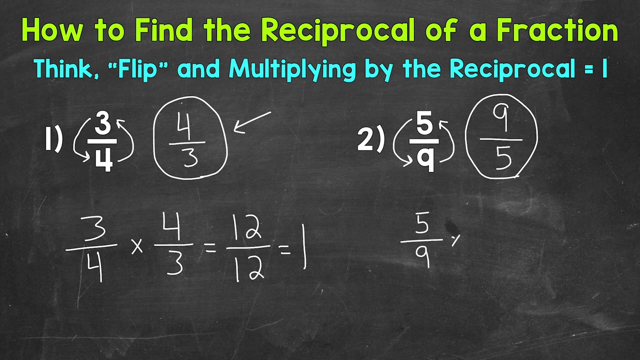 The denominator, the 9, is going to become the numerator and the numerator of 5 is going to become the denominator, So we get 9 over 5, 9 fifths. Let's multiply our fraction 5 ninths by the reciprocal 9 fifths to show that we get 1 when. 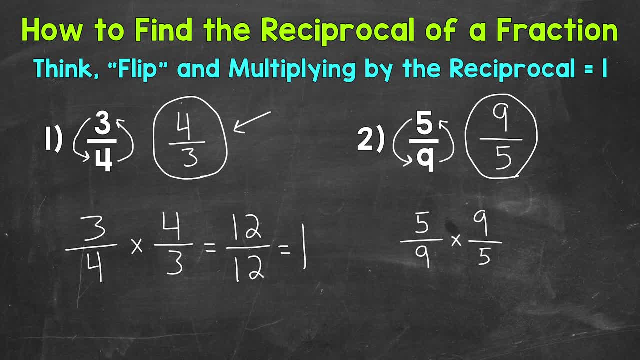 we multiply by that reciprocal. So numerators: 5 times 9, that's 45.. Denominators: 9 times 5, that's 45. Same numerator, same denominator, that equals 1.. So again, the reciprocal of 5 ninths is 9 fifths. 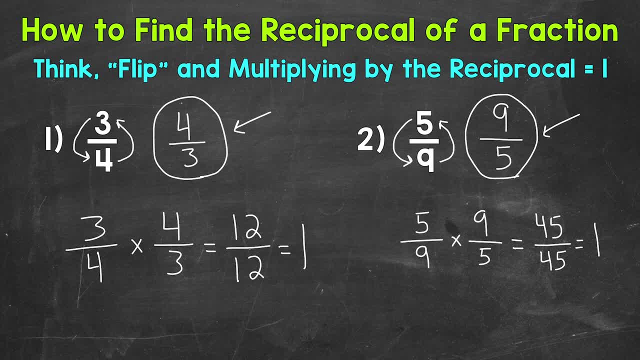 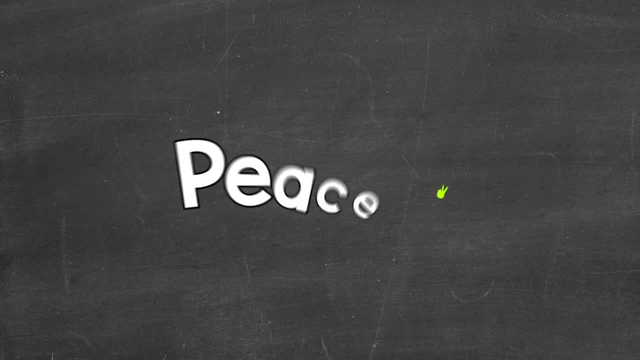 So there you have it. There's how you find the reciprocal of a fraction. I hope that helped. Thanks so much for watching. Until next time, peace.